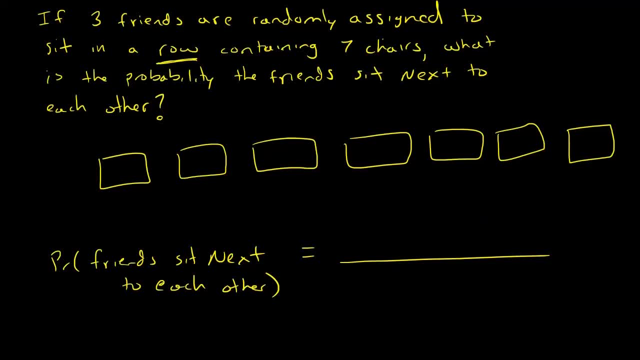 doesn't really matter. We just care about whether or not they're going to sit next to each other eventually. So we don't want to use a permutation, we just want to use a combination where you have the order of them sitting in these chairs. 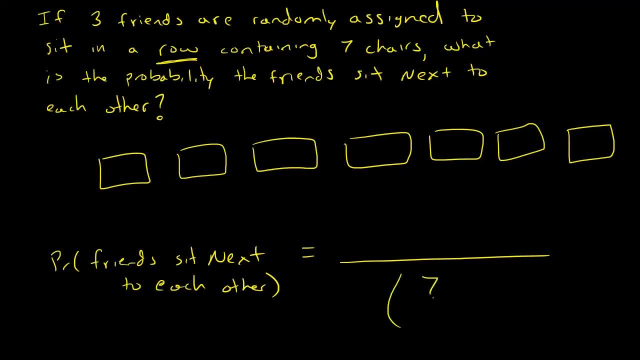 it's irrelevant. So, basically, we have seven chairs and we are choosing three for the friends to sit in. Okay, so what about how many ways in the numerator we need to think of? how many ways can they sit next to each other in this row? 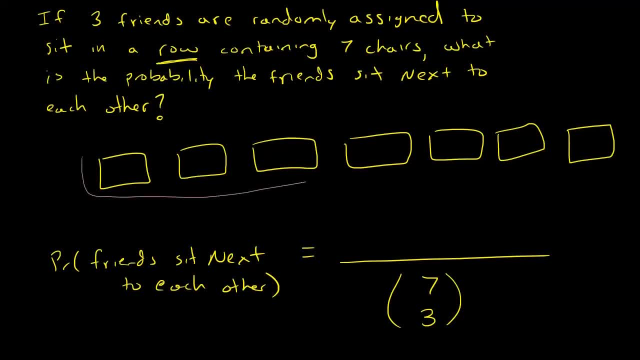 So let me see they could sit next to each other. if they're assigned to sit in these three right here, They can sit next to each other. let me use a different color if they're assigned to sit in these three right here. 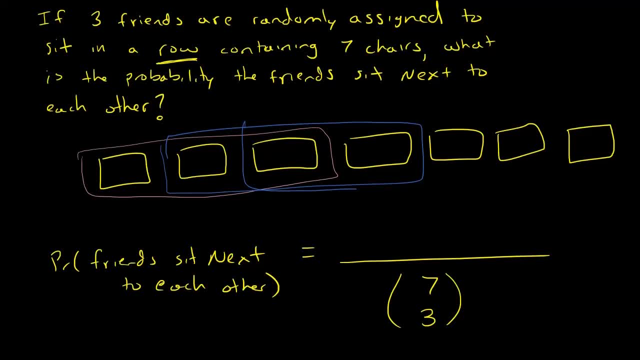 They'll sit next to each other if they let me use a different color. if they sit in these three chairs right here, they will sit next to each other. if they sit in these three chairs right here. And, lastly, they will sit next to each other if they sit. 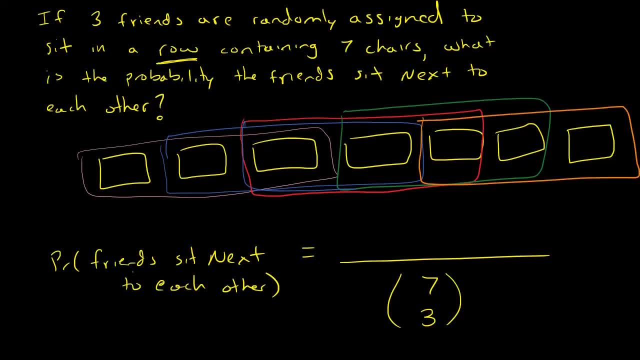 in these three chairs right here. okay, and that's the total number of ways that they can sit next to each other. so how many ways was that? there's one, two, three, four, five. right, there are five different ways that the three friends can sit next to each other, so that's five. 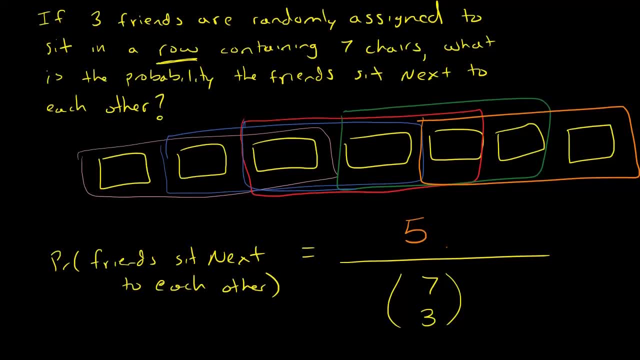 in the numerator. okay, in general, in general, the total number of ways you can sit next to each other would just be the number of chairs, right, and then once you get to the end, you see I couldn't. I couldn't say there were six because I ran out of seats, so it would be the number of chairs to say. n is the number. 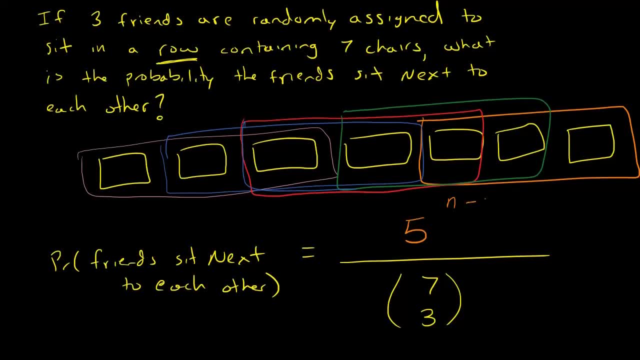 of chairs minus the number of friends that you have. so say, K, we have three friends, that's seven minus three, and then plus one, because the first chair also counts. so you so seven, seven minus the three friends, plus one, which is five. right, you can also, just like I said, just kind of count through it and think it through, you know. 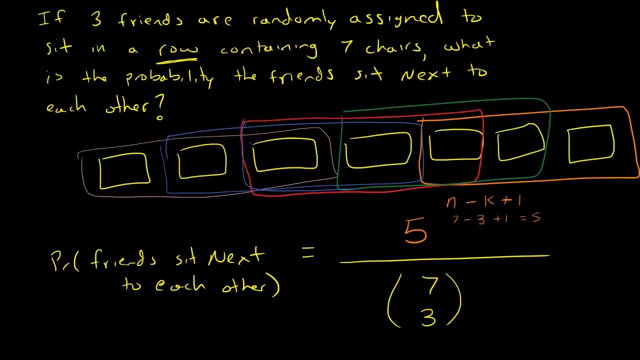 by, by just seeing how many ways that you can sit together, right, but if you have much, much more chairs or more friends and in general, this is the formula of how you arrive to that five here. okay, so now, how do I calculate this? um, let's see, we would have five in the numerator and the denominator we have. 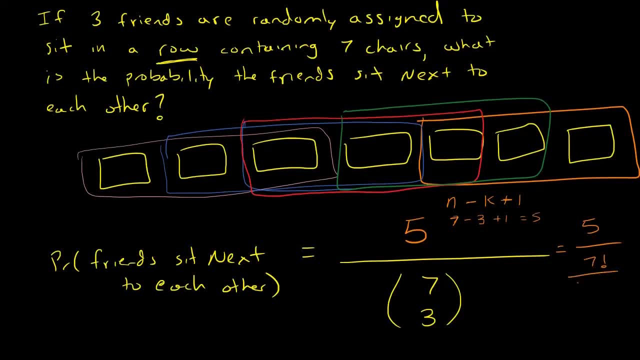 seven choose three. what a 7 choose three. that is seven factorial over three factorial 7 minus three factorial right, so that is 5. let me go ahead and scroll down here, so I'm not room. so that's five over seven factorial, three factorial. so that is is five. let me go ahead and scroll down here. see it now? let's help me out. 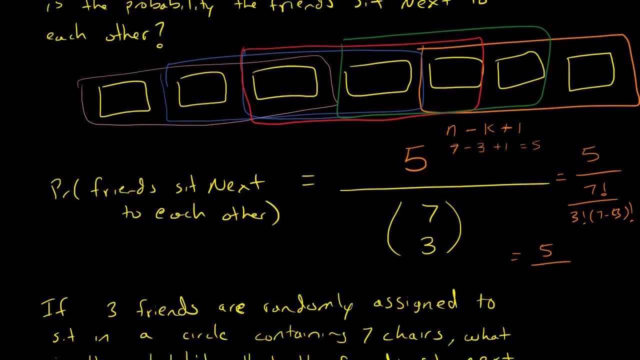 Okay, so this is just one of the order three and nonpermanence, and that's five over. now Let's see how this works. That really does work. I can snap, because this is the log and then I repeat what the machine says the classroom is saying. so these are examples, just like I said. All right, so this is just something I have. the absolutely kan Beef has done every year, but I've kind of forgotten this behavior. Okay, but I kind of forget because I'm just missing something. 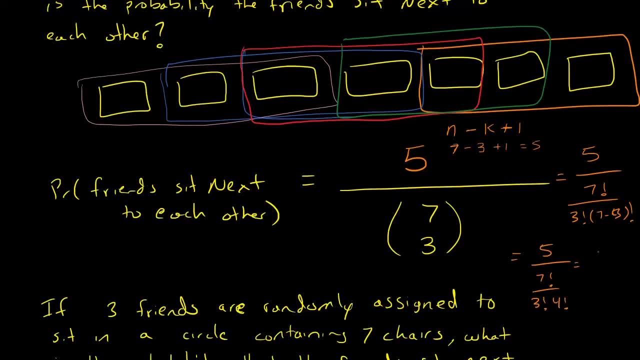 3 factorial, 4 factorial. 5 over 7 factorial- well, that will cancel. so I'll have 7 times 6 times 5 time and then if I have times 4 factorial, they'll cancel with the number with that 4 on the bottom. so then I'll have 3 times 2, okay. 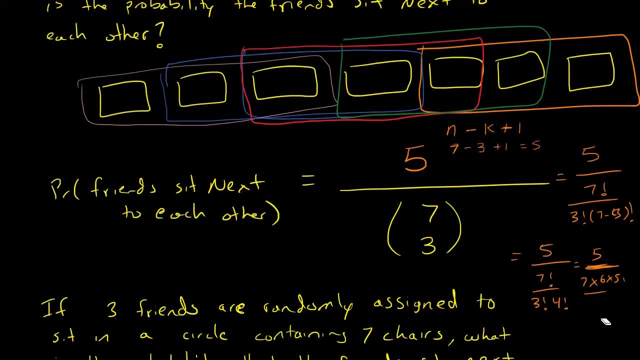 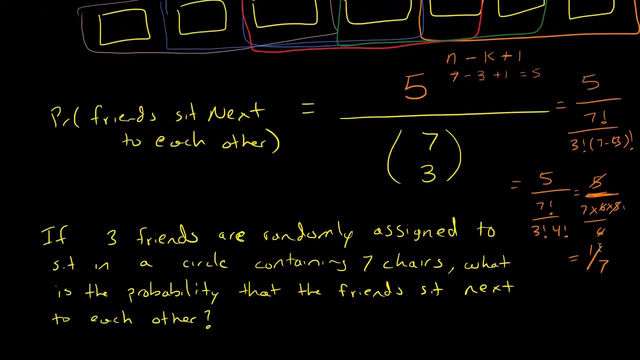 which is 3 times 2, is 6, so that's 6 cancels, and you're left with 7 times 5. that well, the 5 cancels, right, and so you're left with what? is this? 1 over 7? okay, all right, let's see. making the problem slightly more difficult is when 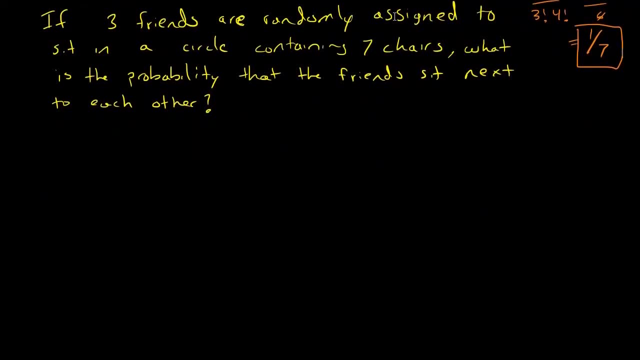 you have the, the, the chairs in a circle. it's really not that much more difficult, but just slightly. so let's go ahead and draw out the problem and draw out the problem, and draw out the problem and draw out my seven chairs. so 1, 2, 3, 4, 5, 6, 7, right, and so now I want the three. 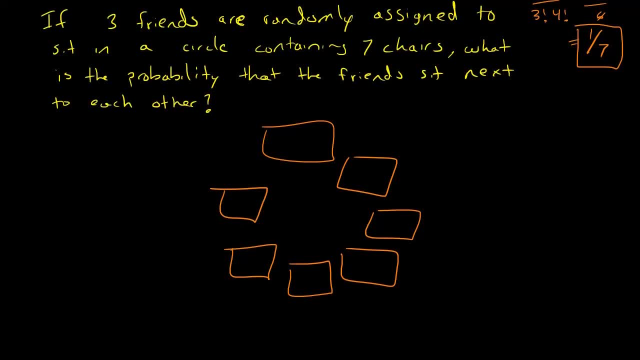 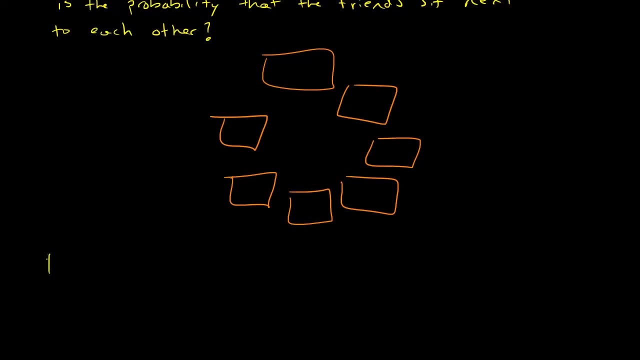 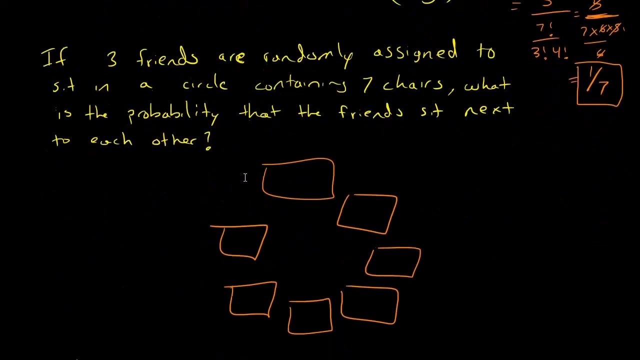 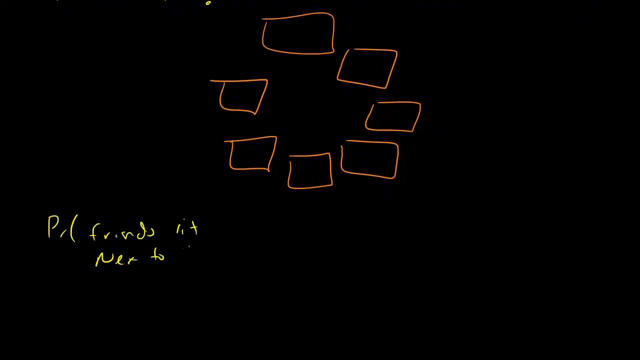 friends to sit together in a circle. okay, once again, you just kind of have to think through. so well, let me go ahead and first right. so we were trying to find the probability that the friends- friends sit next to each other, friends sit next to each other in circle. all right, the denominator again. we still. 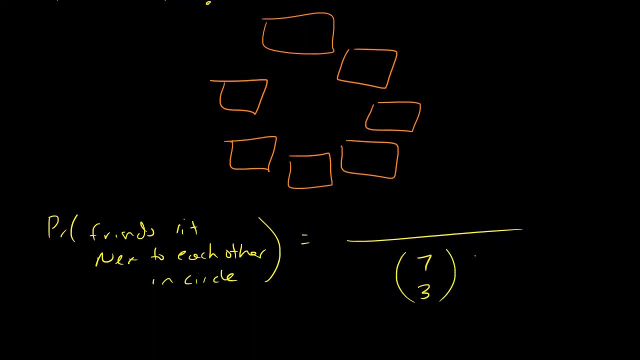 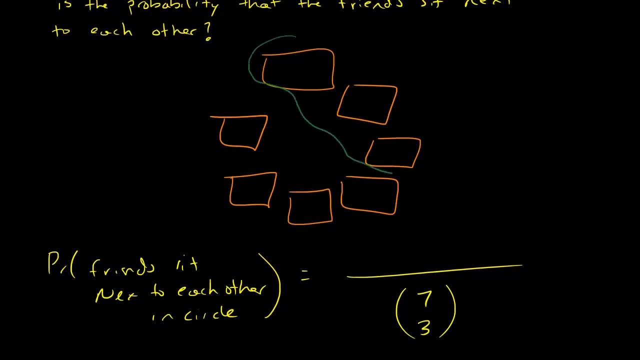 have seven chairs and we are choosing three of them. so the harder part is the numerator right. how many ways can these three friends sit next to each other? so they will sit next to each other if they select these three right. they will sit next to each other if they select these three. 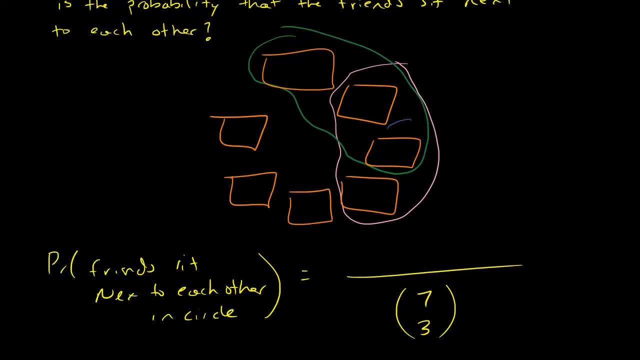 they will sit next to each other if they select these three, okay, and you might see the pattern and be able to figure out what this is going to be. oops, I missed one, so let's see these three. okay, then we have what we have, then we have these three and we have. 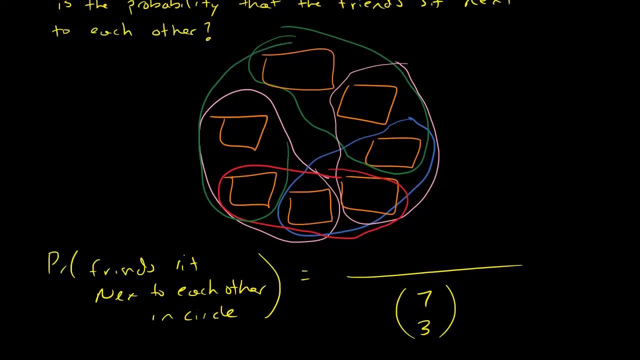 so I just did this once, now I do this one, okay, so basically, every chair gets to be the starting point. okay, every chair gets to be the starting point, and then I get to pick the next three. right, that's basically what I just did: every chair gets to be the starting point. so that means that there are seven total. 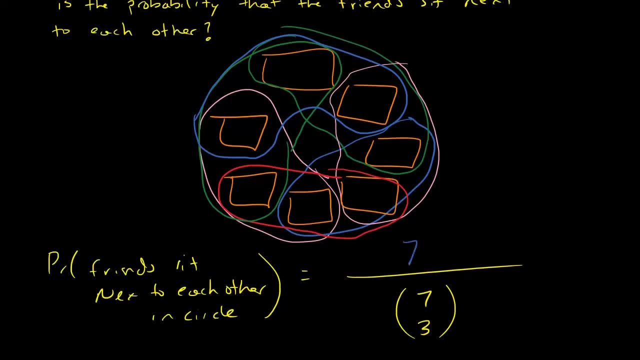 ways I could have made that happen. okay, every chair was the starting point, so there's seven total ways that the three friends can sit next to each other. they can either start here right and select this one, this one, this one. they could start at the second chair and I've sat- and this one, this one, or this one. they 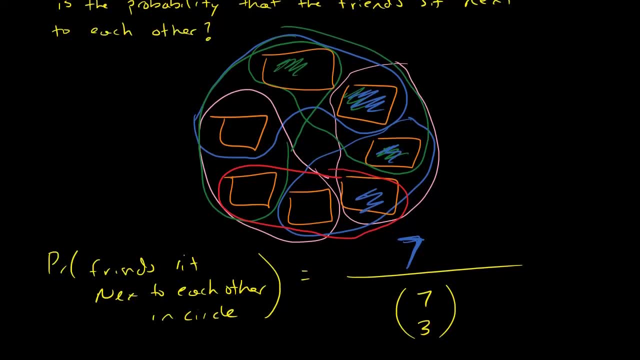 could start at the third chair, and I've sat here here. here they could start at the fourth chair right, etc. so every, every chair gets to be the starting point. so that's why we have seven in the numerator, seven different ways that three friends could sit next to each other right, and then once again, we can.